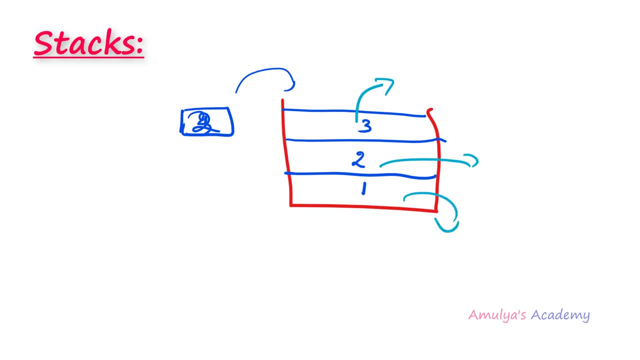 one, next second, one, next first, one, right. so this is the last in, first out principle, and stack works based on this concept. now let's see the basic operation performed by the stack. the first operation is push, second operation is pop, third operation is peak or top, and 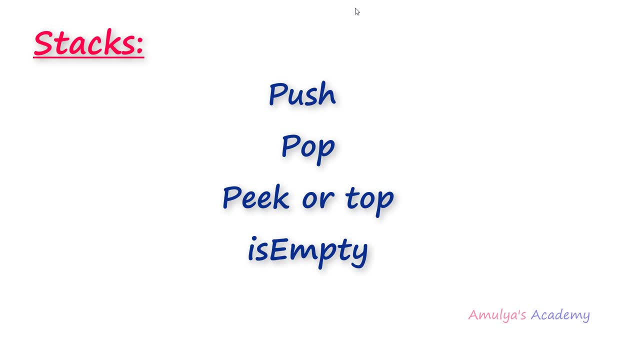 the fourth operation is isEmpty. Push operation adds the element to the stack. if you want to add the element to the stack, you need to use the push operation. pop operation will remove the element from the stack. peak or top will give you the element which you. 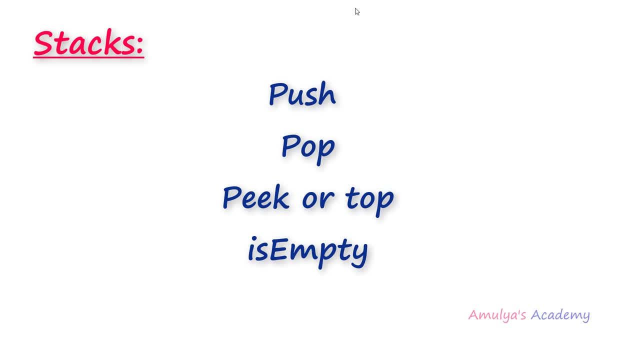 is present at the top and isEmpty is nothing but which will tell you whether stack is empty or not. So in this operation, push and pop operation is very important. So i'll explain you this two operation with example. So first let's talk about the push operation. 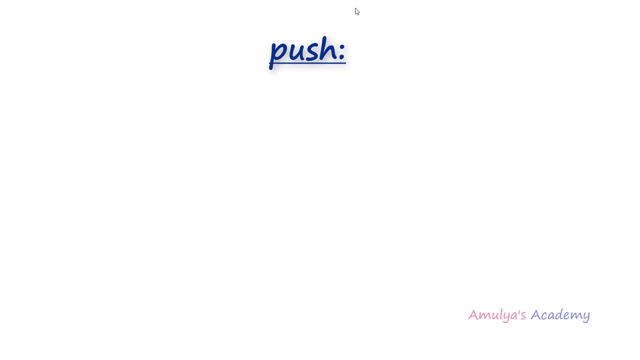 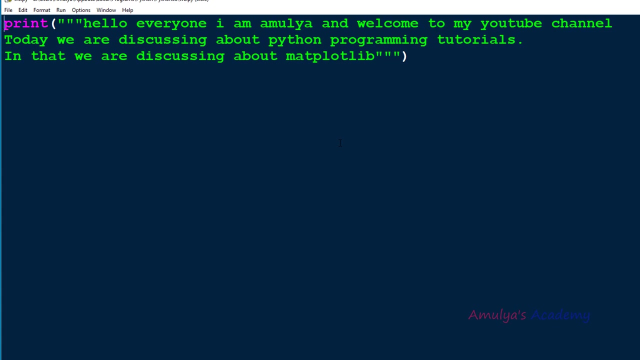 So, as i said, push operation allow us to add the element to the stack. So let's take the example for this. Let's take an editing file example using the undo features. Alright, so i'll take a python file here and in the python file i have a print function. 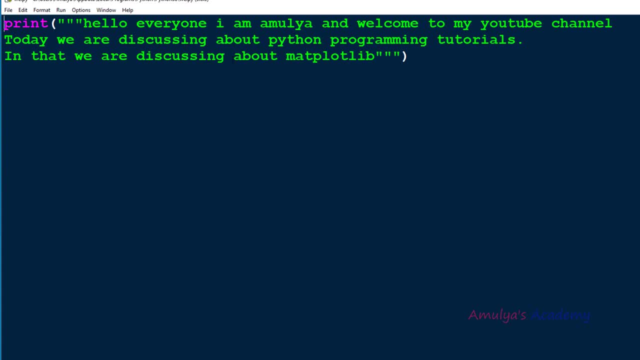 and i have few statements. ok, Now, if i want to remove any word from here. for example, i'll remove this word about: ok, When i delete this now, about word will be added to the stack using push operation. Next, i'll delete amp. Ok, now, amp will be added to the stack using push operation. 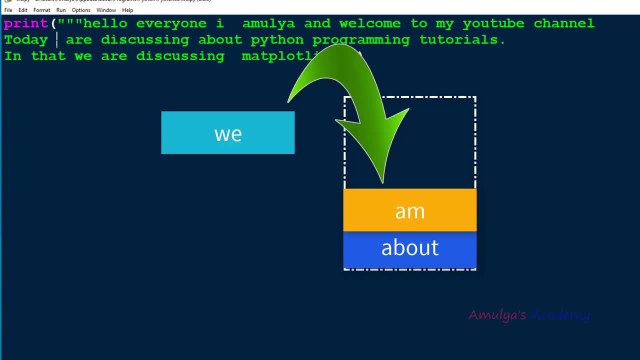 Next, i'll remove v. Now v is added to the stack using the push operation, right? So this is about the push operation, which allows us to add the element to the stack. Now let's talk about the pop operation, which is also very important operation. 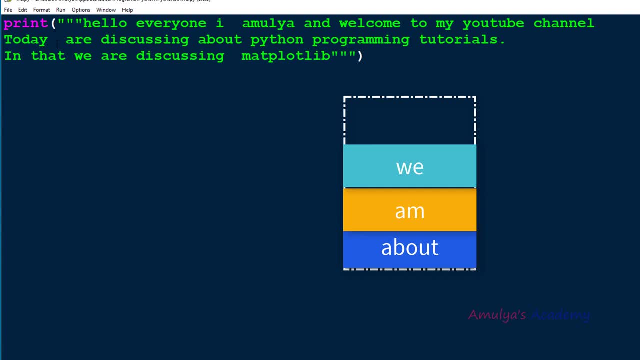 In the pop operation. it will allow us to remove the element from the stack. Ok, So let's use control z now. that is the undo operation First. the element which we deleted last, that is v, will be removed first. So when i press control z, here we here. we can see v is appeared here first. ok,